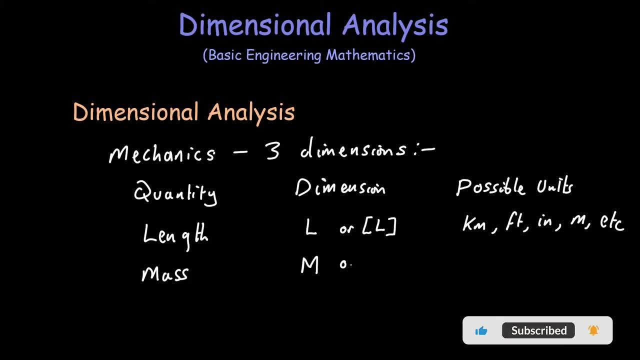 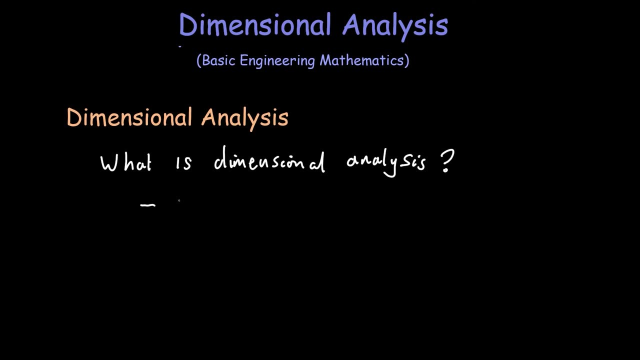 which we can represent as capitalized L, M and T respectively. So what is dimensional analysis? Dimensional analysis is simply a procedure used to test the validity of an equation or to help us derive new equations. So this question states: show that the expression V equals AT is dimensionally correct. 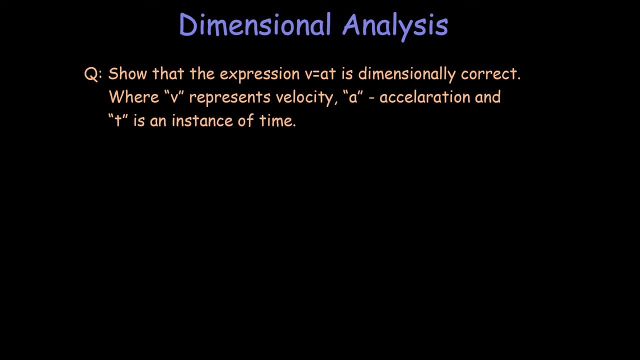 where V represents velocity, A acceleration, and T an instant of time. So our goal here is to show that terms on both sides of the equation have the same dimensions If we choose to use the International System of Units or the SI units. 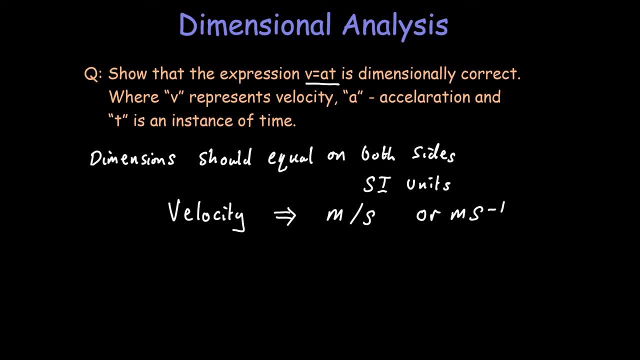 velocity has units of meters per second. Although the choice in unit in dimensional analysis doesn't matter, we could quite easily express velocity as miles per hour. The point to notice here is that the velocity can be expressed dimensionally as a length over time. 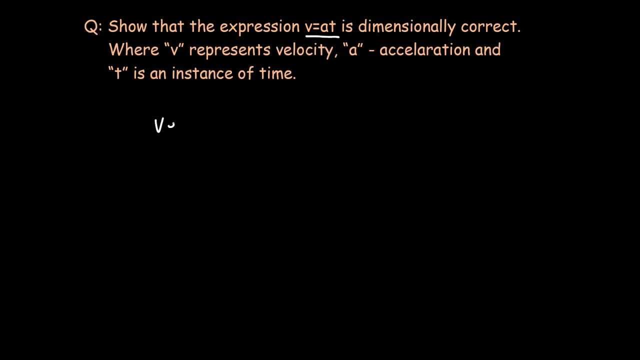 And to find the dimensions of acceleration we follow a similar process. Acceleration has dimensions of meters per second squared, and this is expressed as length over time squared. The instance of time has dimensions of time T. If we now plug these dimensions into the expression, V equals AT. 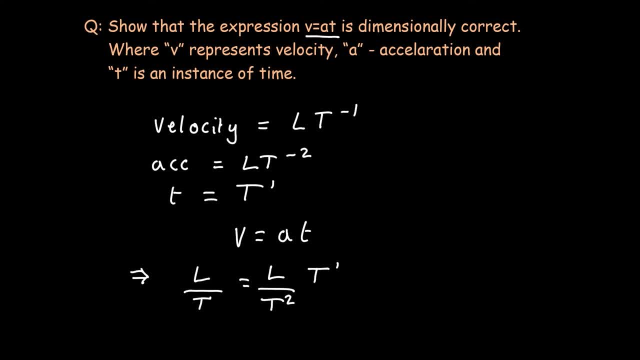 we can see if they balance on each side of the equation. On the right hand side of the equation we can cancel out T in the numerator and one of the Ts in the T squared in the denominator. We end up with dimensions that are equal on both sides of the equation. 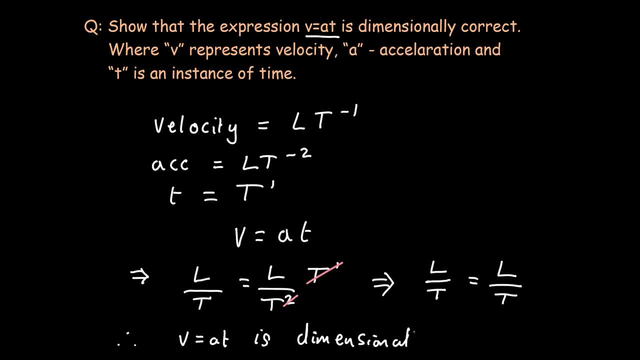 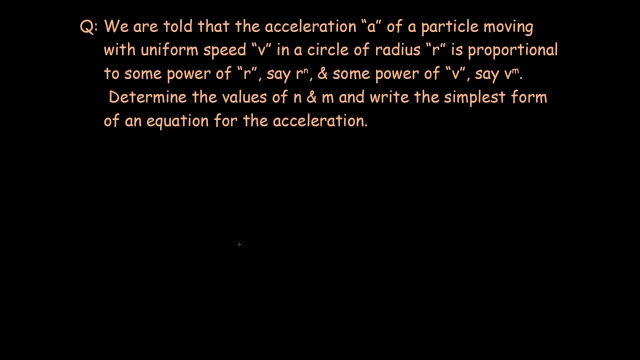 In other words, the expression V equals AT is dimensionally correct. We are told that the acceleration A of a particle moving with uniform speed. V of radius r is proportional to some power of r. say r to the power of n and some power of v. say v to the power of m. Determine the values of n and m and write. 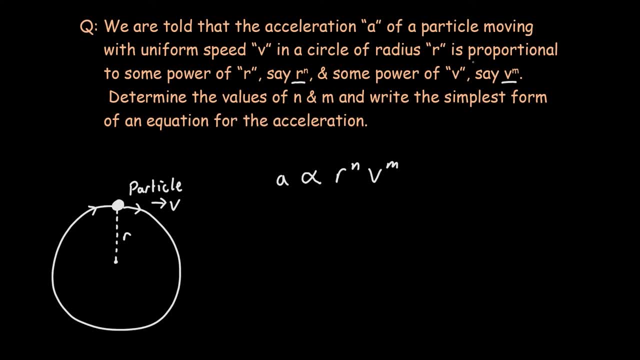 the simplest form of an equation for the acceleration. Let's first write acceleration as a proportional to r to the power of n, times v to the power of m. We can rewrite this with a constant of proportionality. From the last question we found that the dimensions of velocity and acceleration can be: